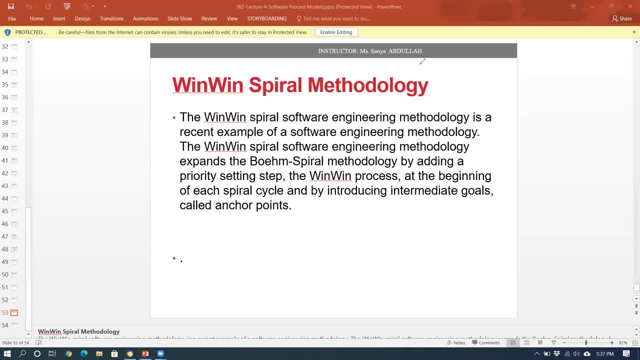 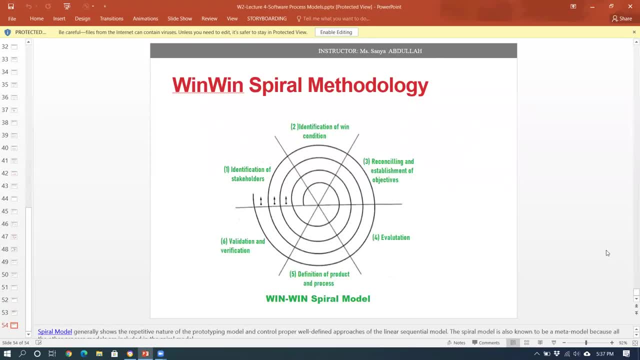 That we are going to move or proceed into this spiral methodology. Okay, Now the activities that were involved in it. we have already seen. Okay, And what were your activities? That at the start of the spiral, what are you doing? 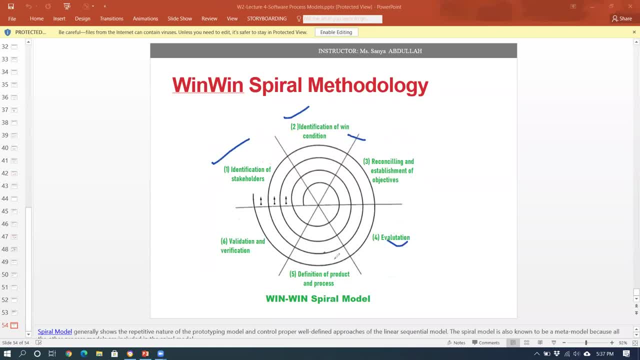 The first, second, third, fourth, fifth, sixth activities that you are adding. Okay, First of all, this is the activity that you have to negotiate with all the stakeholders of your system. First of all, you have to identify them. 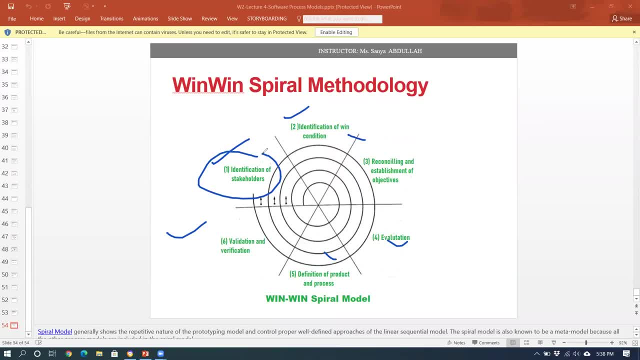 Okay, Stakeholder, So they can be anyone in the organization. Okay Right, Who has a direct business interest with the system you are going to make, the product you are going to make? Who has a direct business interest with it? 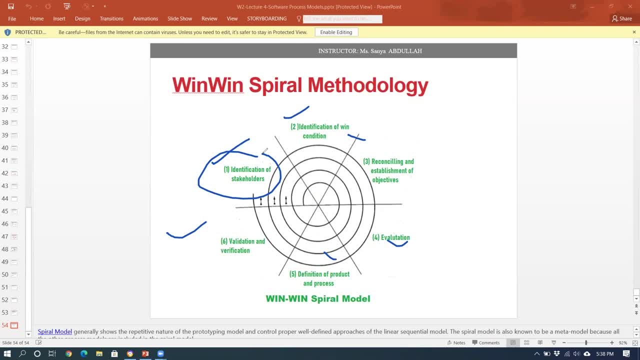 Okay, And somehow that person has to either use it, or if that system is successful, then it will have an increase in its shares on a particular end, Or he will get some reward, Or if it fails, then it is definitely a matter of loss. 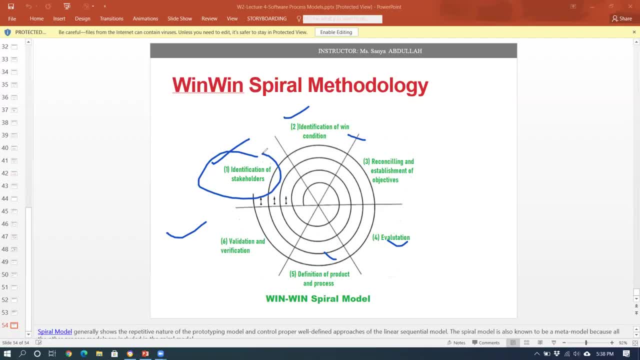 Okay, So somehow that same thing will be criticized or there will be a discussion on it. So the stakeholder could be anyone in the organization whose particular product has some direct business interest. Okay, So you have to identify. After that, when you have identified the stakeholder, then it is definitely a matter of what the next thing he says to you. 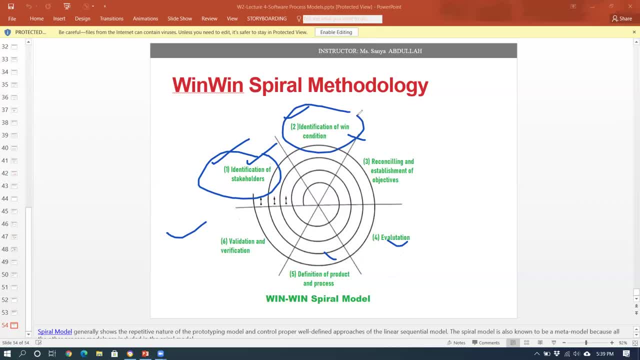 That you have to see the win conditions. Okay, What will be the win conditions? Obviously, we have to keep in mind the things on which the interest of your user lies. The user who is your system owner, the one who is making you, he tells you that these things should happen. 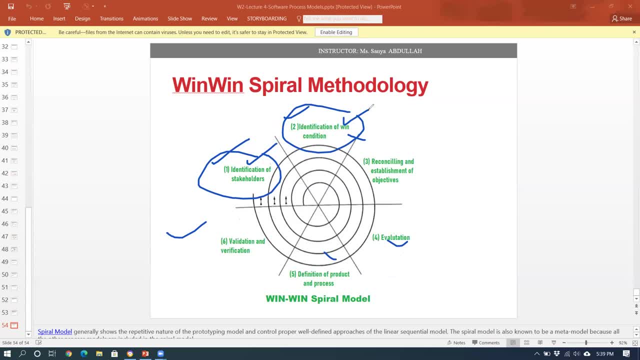 This is my interest. So you have to, you know, identify those conditions that your customer is keeping with you And those conditions that you are making the developers somehow, with the possibility that this can happen and this cannot happen. Okay, So what you have done, you have to reconcile with win conditions. 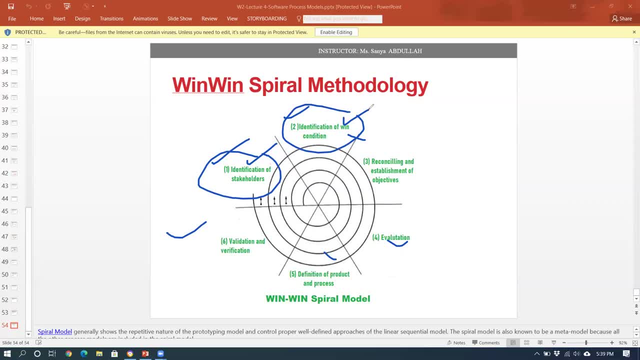 How will you do it? Obviously, these things will not come down from the sky Or it is not written anywhere. There is no document anywhere. There are no rules in the business world. You do these things through negotiation, You do this work through negotiation. 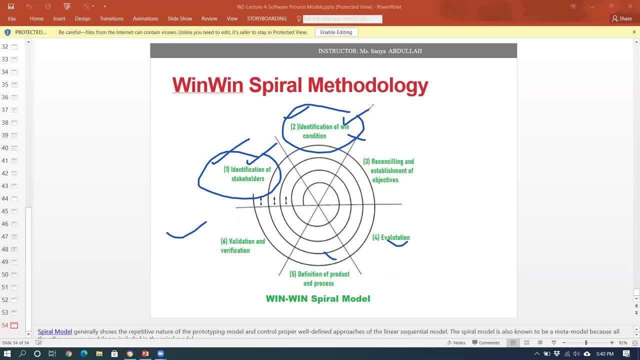 Okay, When you will negotiate, you will listen to some things in negotiation, You will tell some things about yourself And at the end you will come up with such a set of objectives. You will make such a set of objectives, Okay. 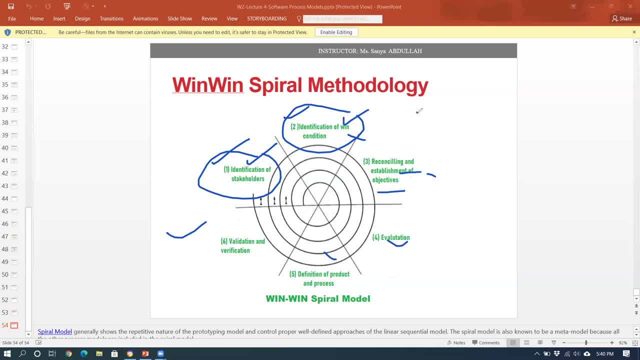 Which are mutually satisfactory, On which your customer is also satisfactory. In fact, your stakeholder is also satisfactory. Thumbs up to you And somehow you are okay with that. Okay, Now these things are going to somewhere Possibility. 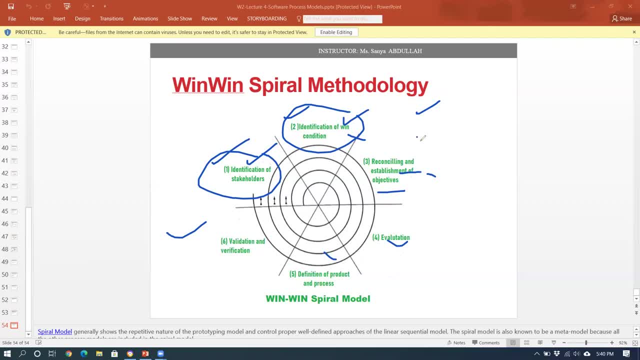 This is what is coming, Okay, So reconciling and establishment of objectives. This means that we have to reconcile win conditions, That which which. How to do it? Remember this: Through negotiation. This is the only way to do it. 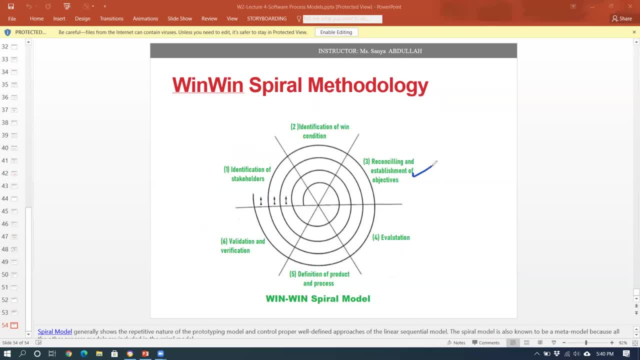 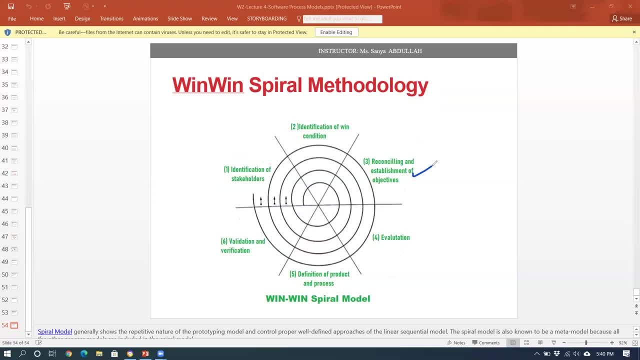 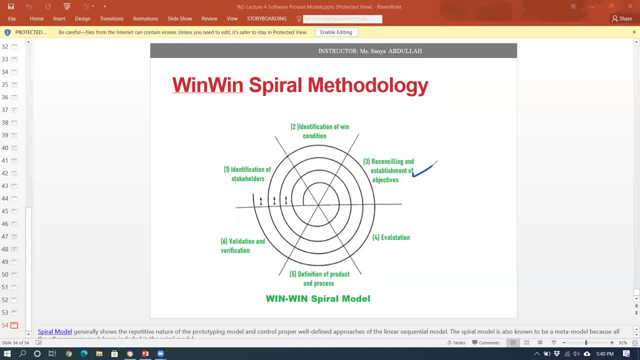 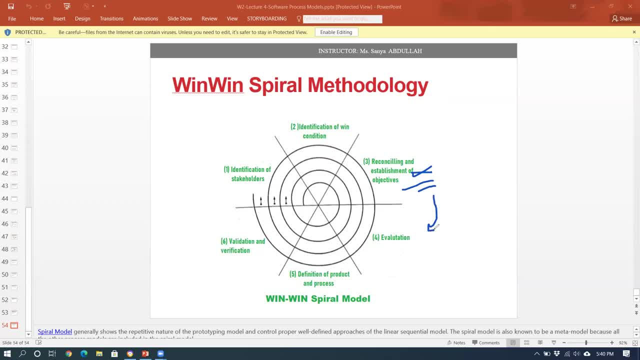 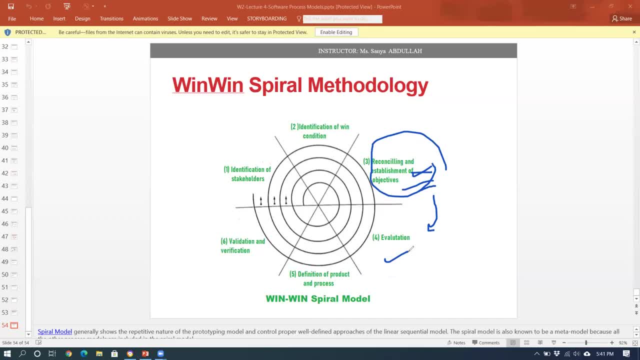 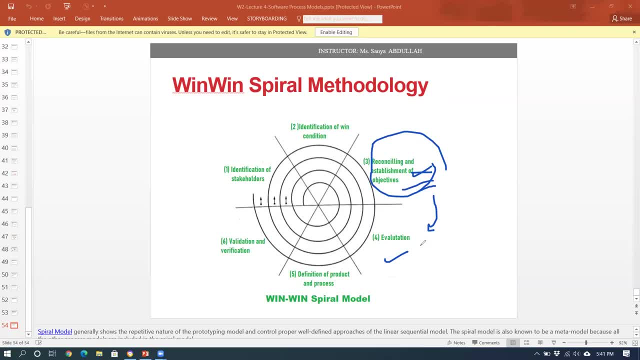 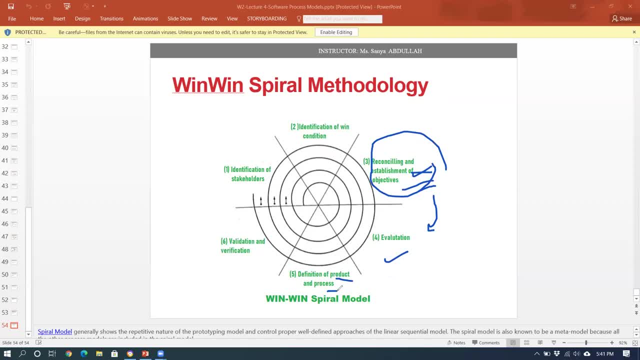 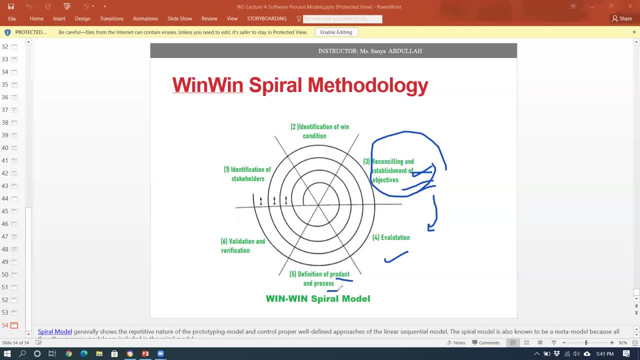 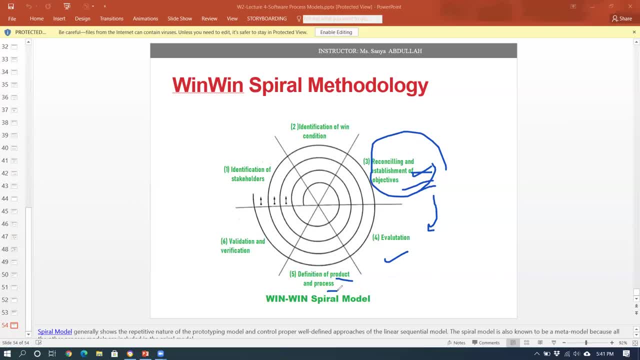 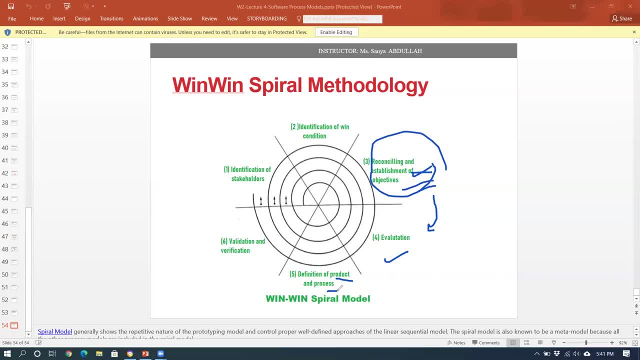 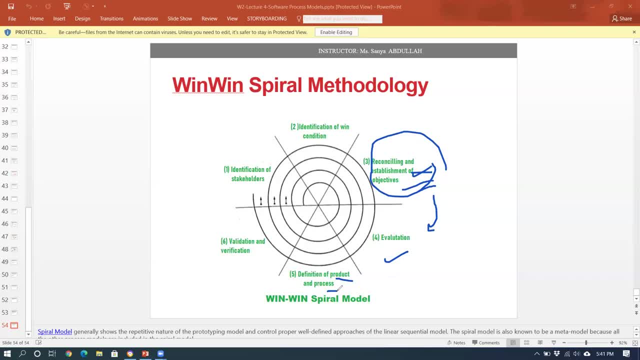 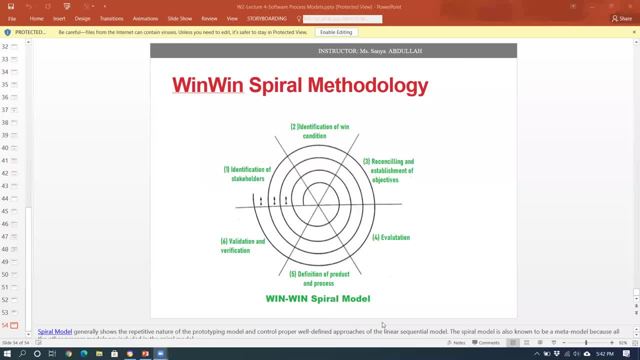 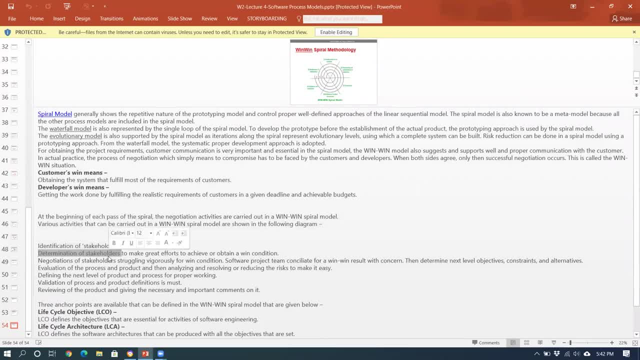 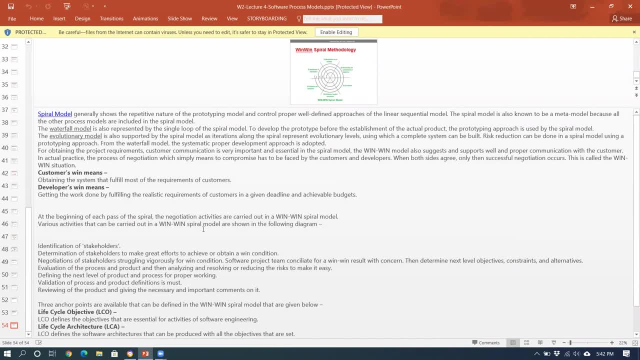 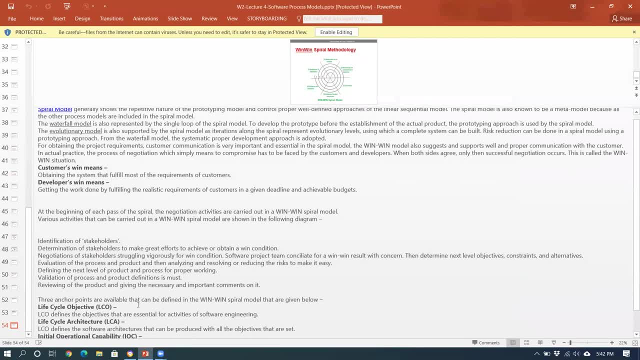 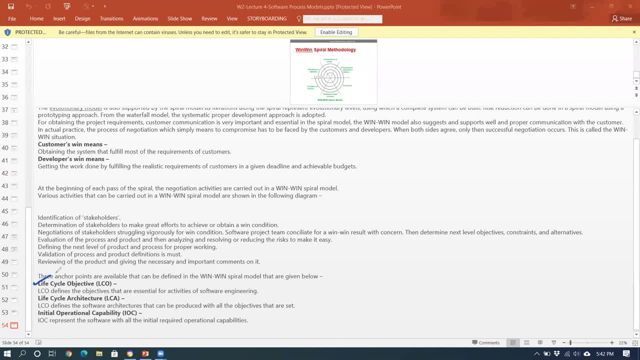 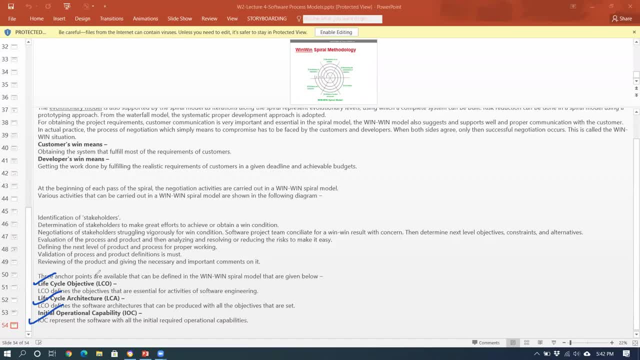 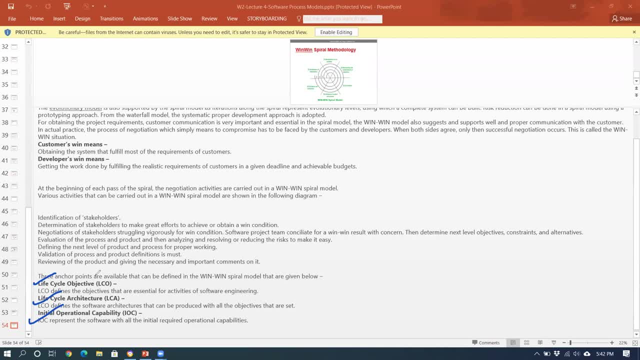 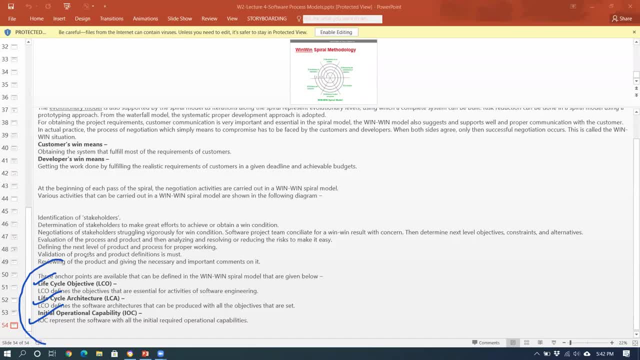 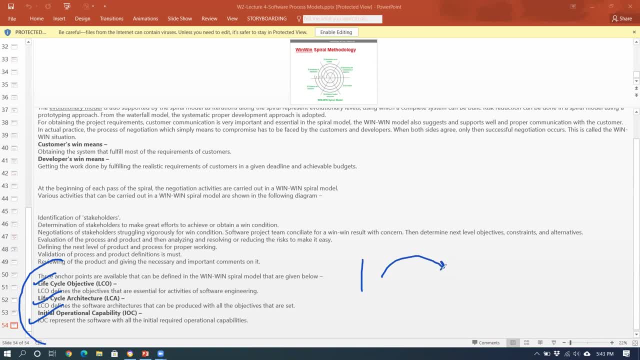 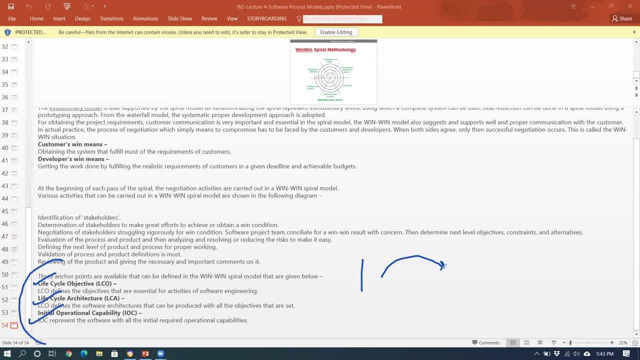 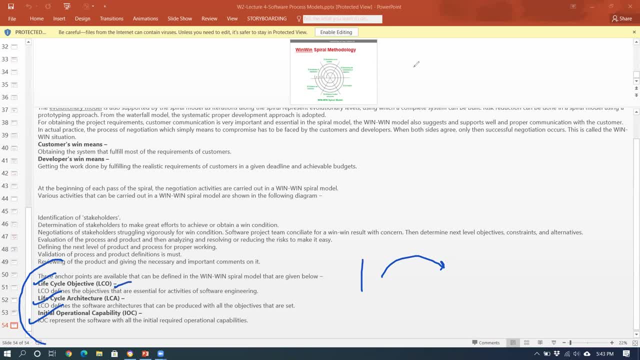 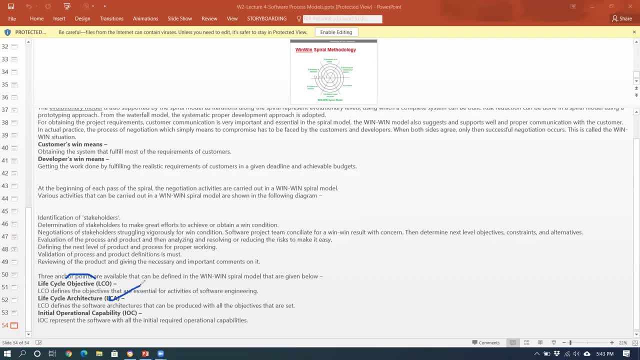 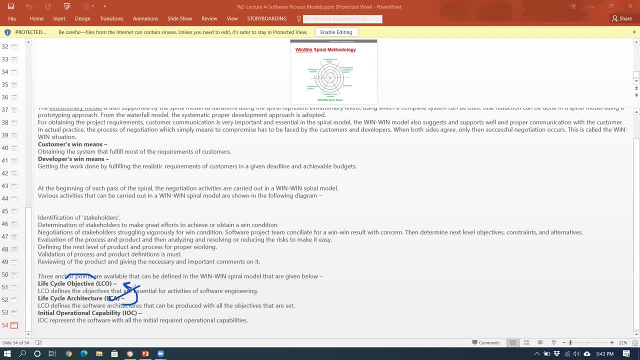 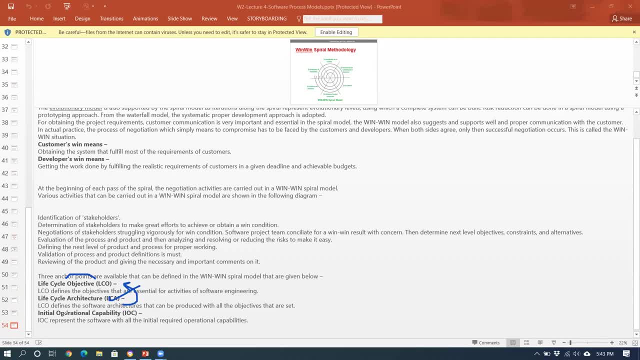 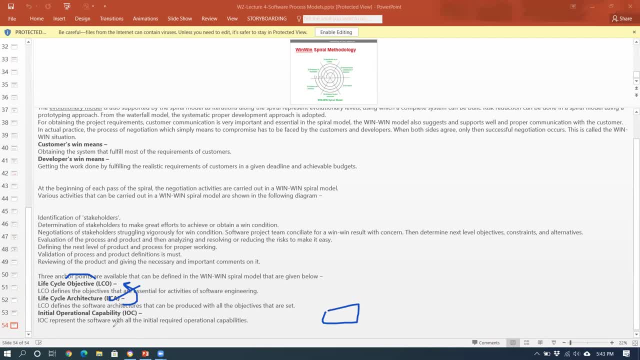 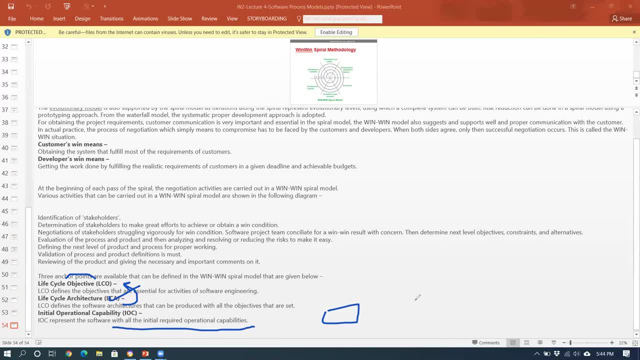 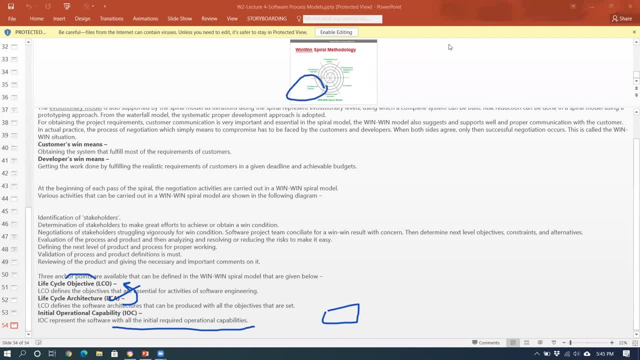 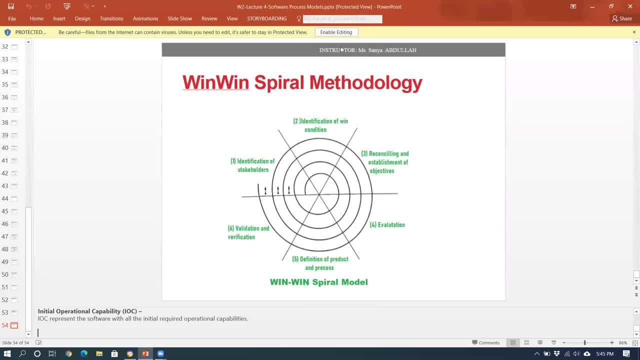 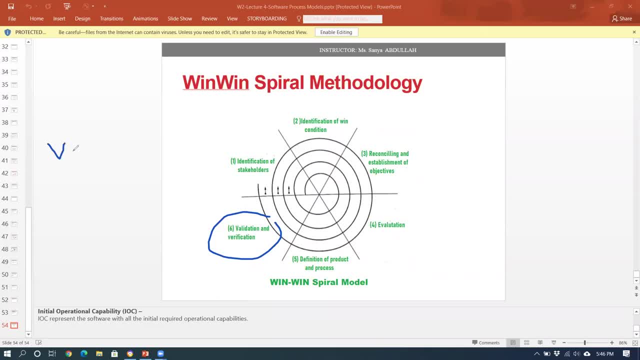 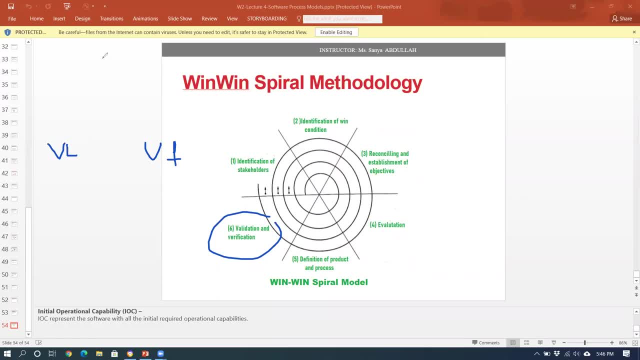 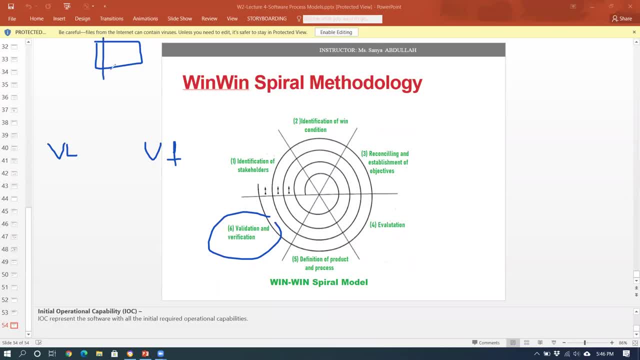 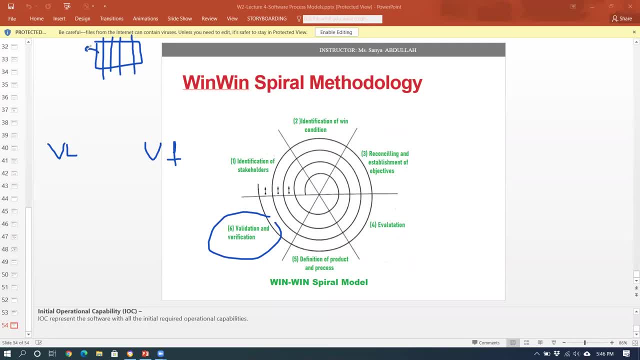 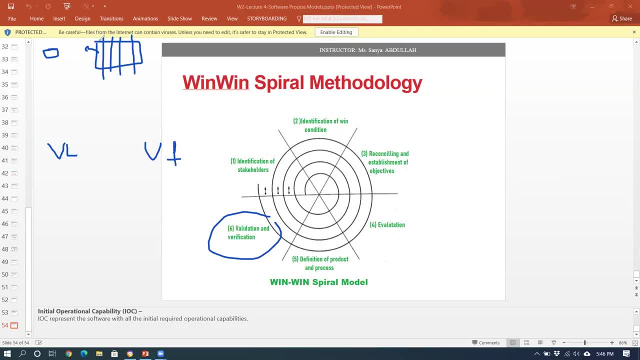 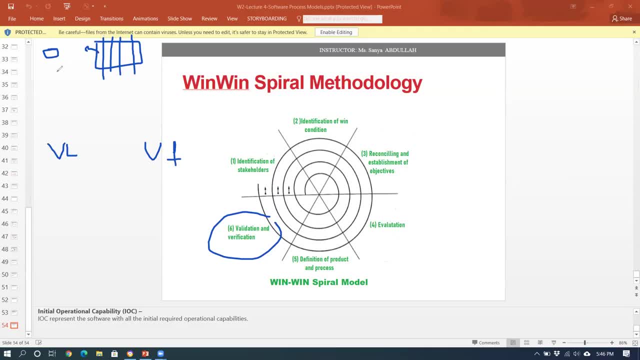 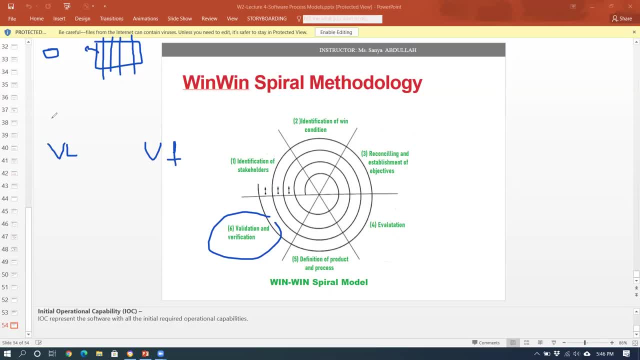 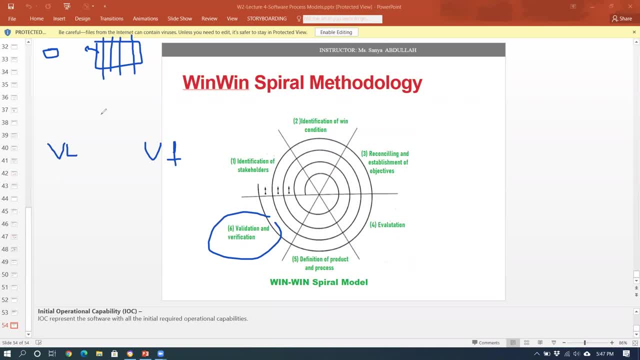 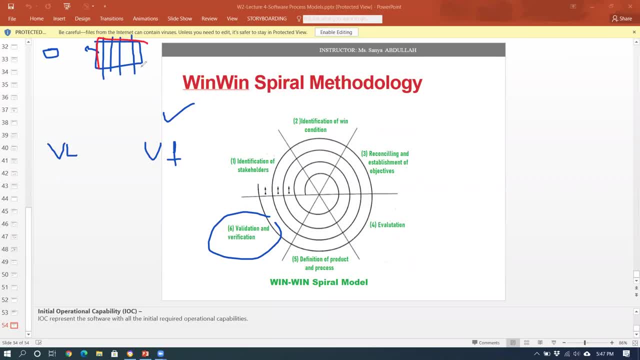 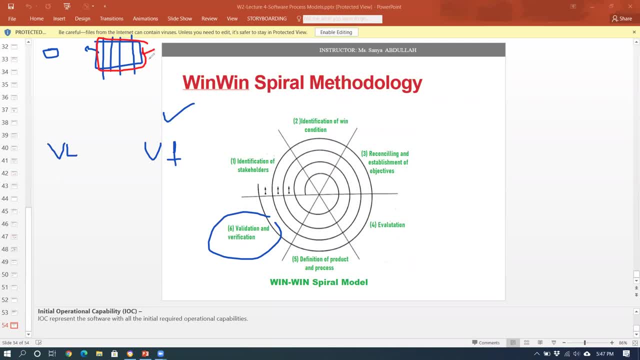 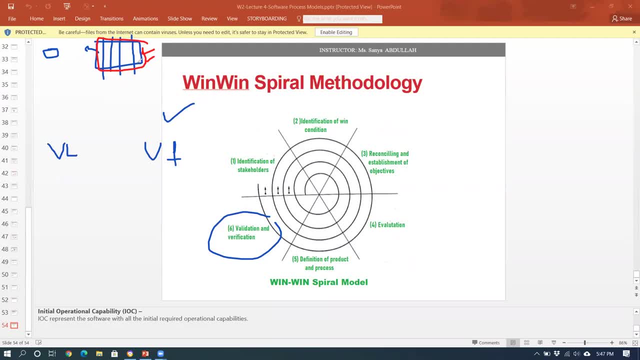 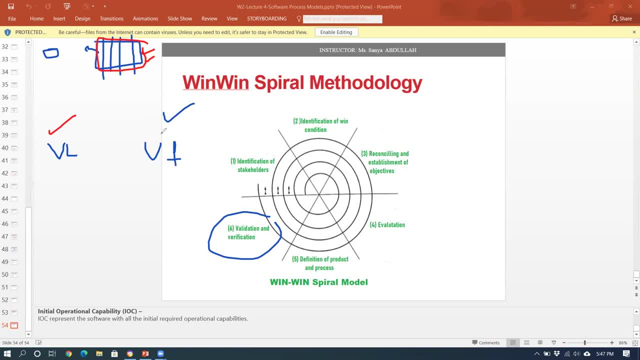 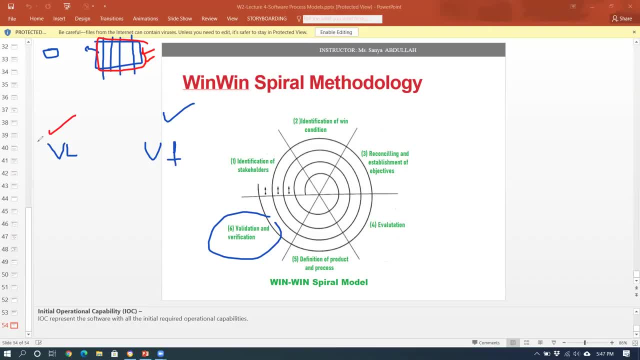 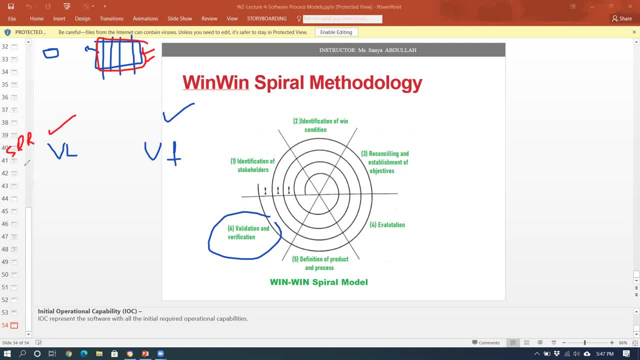 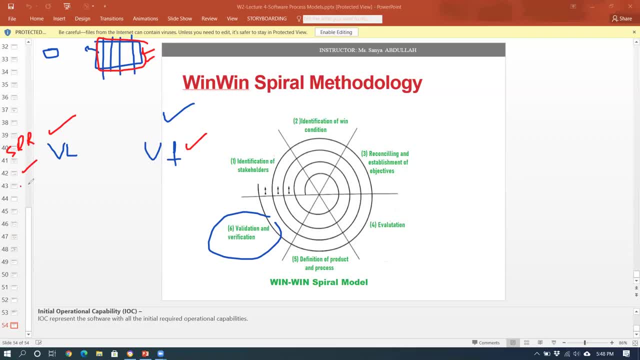 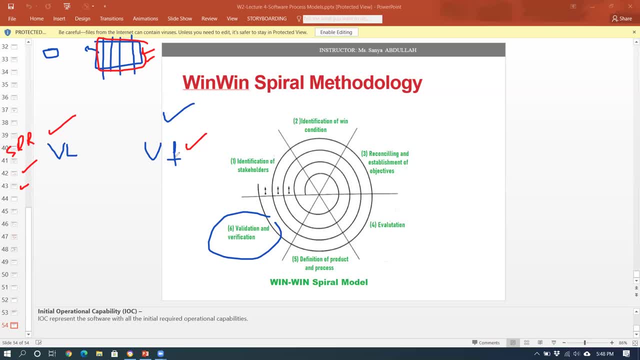 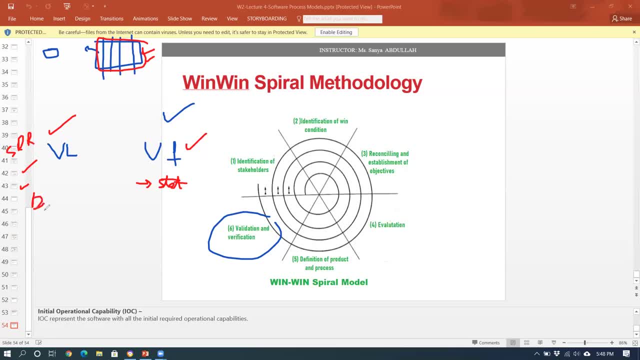 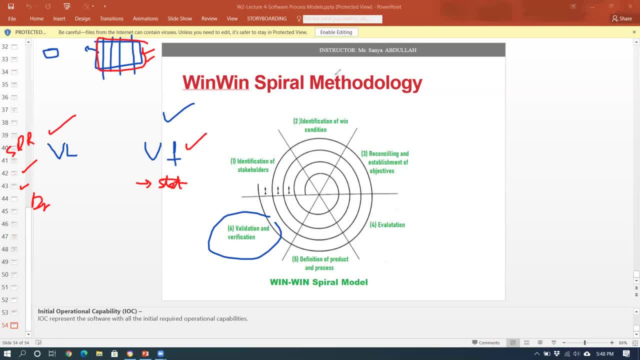 Okay, So this is the only way to do it. Okay, So this is the only way to do it. Okay, To tell you that you are not executing anything over here. you are not executing anything overall. You are just reviewing, For example, my entire program has been created. 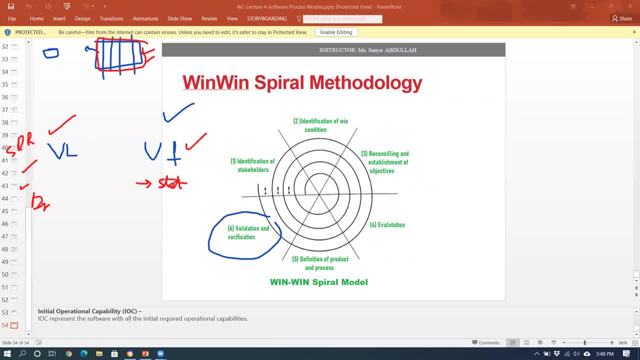 Now I have run it, executed it to see if it is fine or not. No, not like this, Because the phase has been created, you have not executed it. you are just taking a review, Because your entire system has not been created yet, so you will just specify the phases. 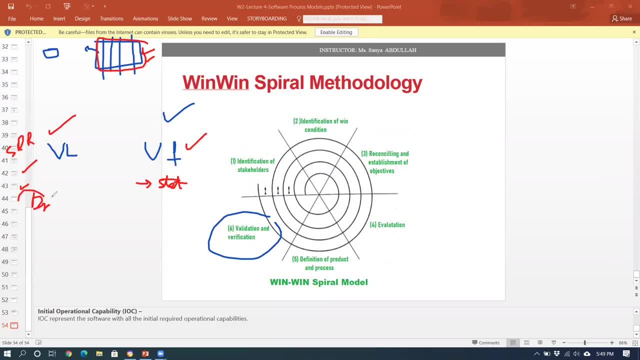 That you are taking the review, whether it is fine or not. Here you are also calling it dynamic, because here you are executing the actual overall system, Whether it is giving the right result or not. So I am going to end it by this thing. 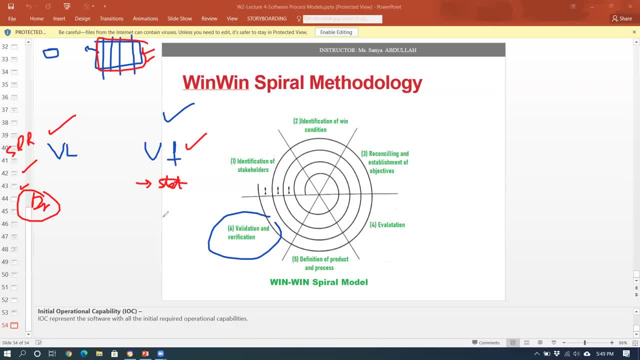 The process of calculating the product during the development is called the verification, And the process of checking the product after the development is called the verification. So I hope that this is complete Now. a lot of concepts have been cleared in your case, So I will wish that you read this PPT with notes: Thank you so much.